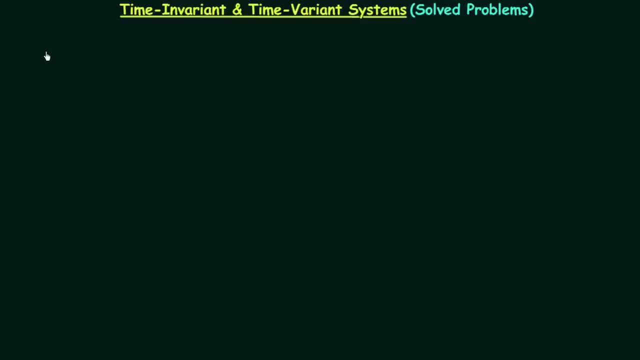 those conclusions. we will try to find out the answers of given questions directly, because when you have multiple choice questions there is no need to follow the conventional method of solution. You can directly choose the correct option by using the conclusions which we will draw in this lecture. So let's start with the first problem. In the first problem, output yt is equal. 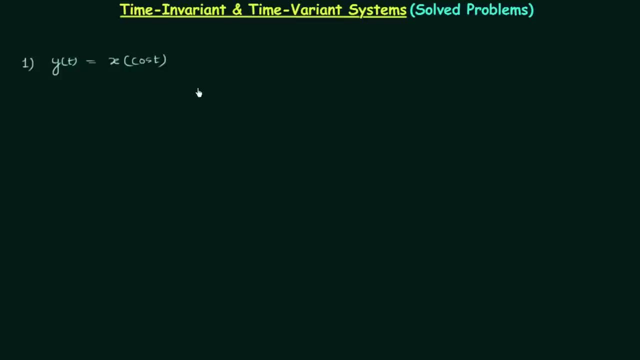 to x cos t. This means there is an input x t, The input is always x t. this is one convention which we are using here. We have drawn the first problem, which is the function output yt, using from the very first lecture of basic system properties, and this input is the input. 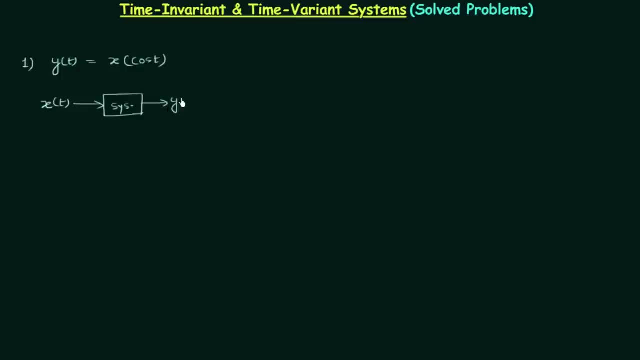 of this system, and this system is giving us the output, yt, which is equal to x cos t, and we need to find out if this system is time invariant or time variant. Now, what do we mean by this statement? the system is time invariant or time variant? this 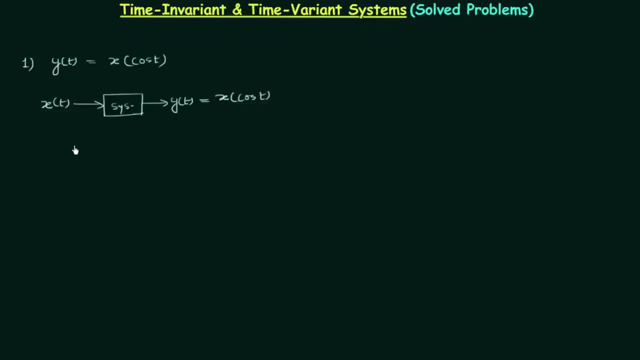 means on providing a delay. let's say the delay is t0. so on providing a delay of t0, we want to check if the system remains same or it becomes some other system. if the system remains same, then it is time. invariant system: there is no effect of delay. and if the system changes, 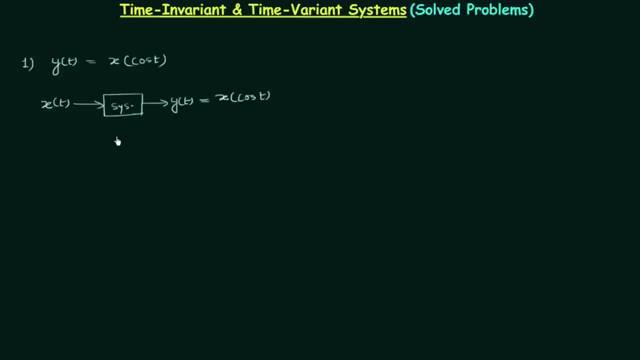 to some other system. then it is time- variant system. So let's see how we can check it. The first step is to provide the delay to the output directly. so we will provide the delay of t0 to the output of the system yt and this will give us yt-t0. so simply replace. 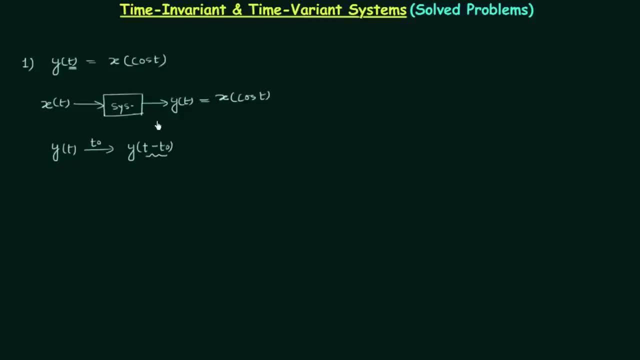 this t here to t-t0. this means we are replacing this t here by t-t0.. So we will have x cos t. This is what we have after providing the delay to the output of the system. Now, in the second step, instead of providing the delay to the output, we will provide the 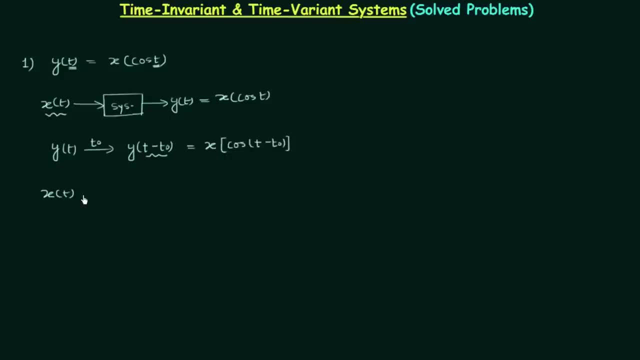 delay to the input of the system. the input is xt and we will provide the delay- the same delay, t0- to the input and we will have xt-t0. now we will feed this to our system, whose property we want to check, So let's feed it to the system. the two systems are same and the output this time we will. 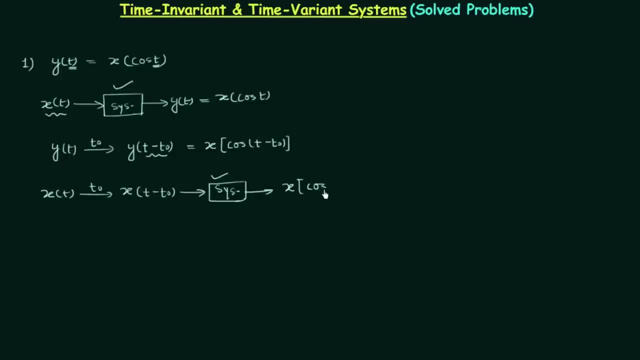 get is equal to x cos t-t0.. Now let's try to understand why we have cos t here. if you see the original system, you will find the input was xt and the output was x cos t. so because of this system, instead of t, 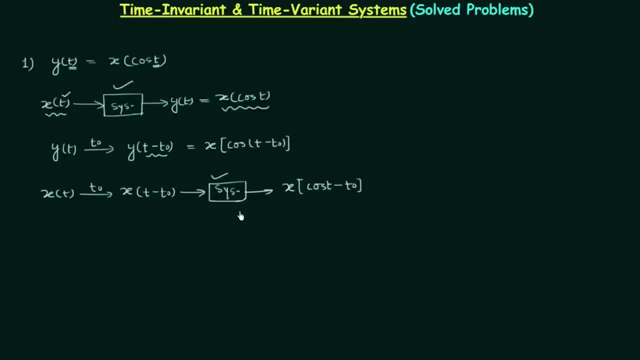 We got cos t, So here what will happen? the system is same and instead of t we will get cos t. This t0 here is a constant, so don't confuse yourself with the variable t. the operation is on the variable t. that's why we have cos t here, and if you compare the two outputs, 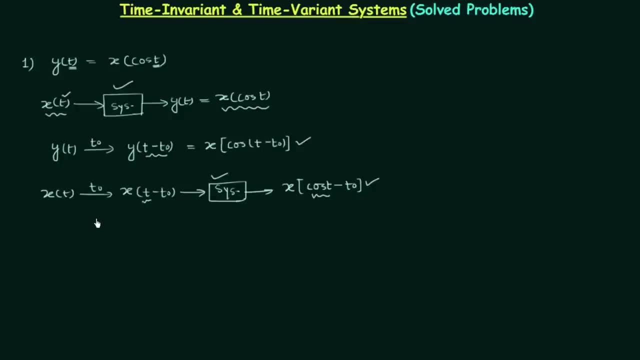 you will find they are not same. This means, after providing the delay, there is variation in the system output. So the system is time variant system. I will write down the answer of this problem. the system is time variant system. Now let's check what will happen if we have an output yt which is equal to x, tan, t. 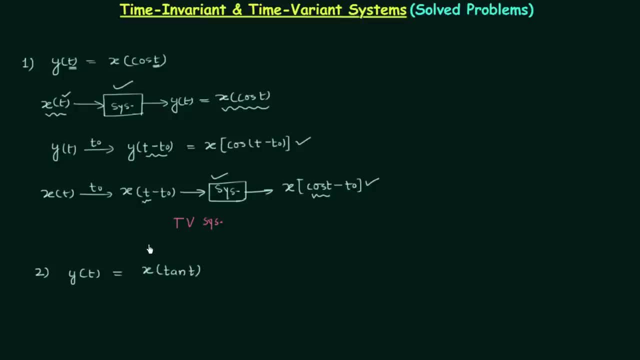 Now there is no need to follow all these steps, because we have already seen: when output is equal to x cos t, the system is time variant system. So this time also we will have the same result: The system is going to be Time varying. 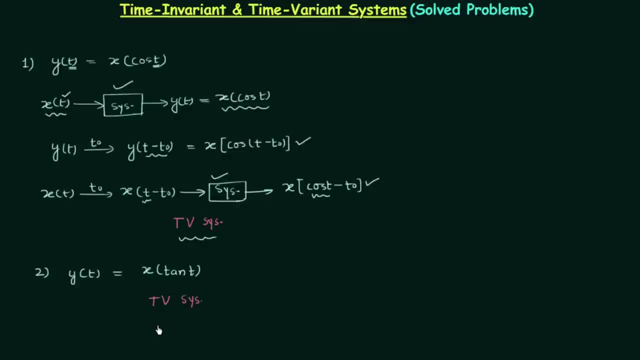 So in this way, you can use the results which we are obtaining in this lecture directly. So we can conclude. we can conclude that whenever there is any time scaling, the system will be time variant and this time scaling is not compulsory to be on the input, it can be on. 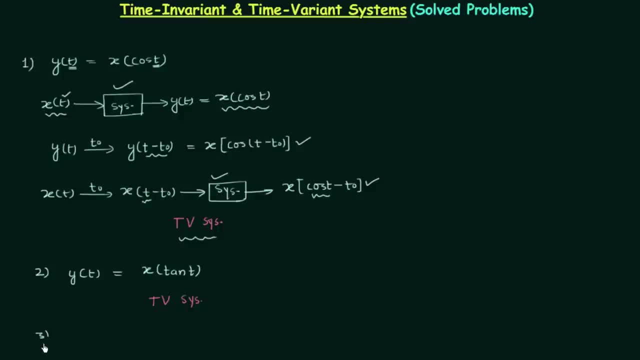 the output as well. For example in the third problem, If we have y t cube and it is equal to x t, then also the system is time variant system. Why time variant system? because there is an operation on the time, which is a scaling operation. 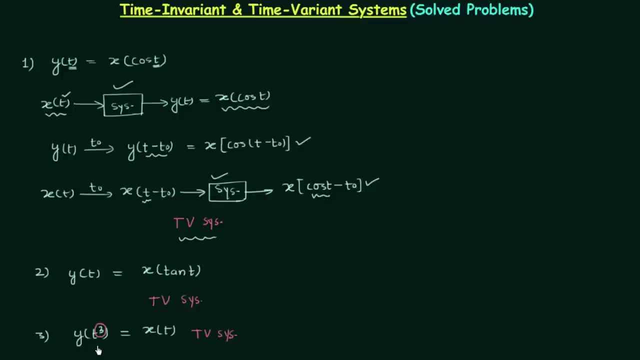 This is not shifting operation, it is scaling operation. That's why the system is going to be time varying system. Let's see few more examples of this in the fourth problem. in the fourth problem the output y- t is equal to x- t square. again there is time scaling on the input side. that's why the system 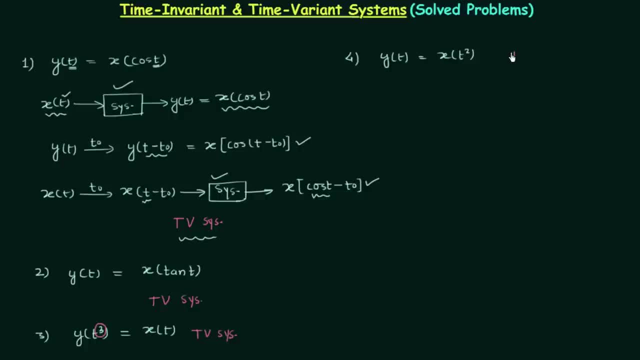 is going to be time varying system. You can check by following these steps. So this is one conclusion which we have till now. Now let's move to the problem number five. and in this problem, Output y, t is equal To cos. 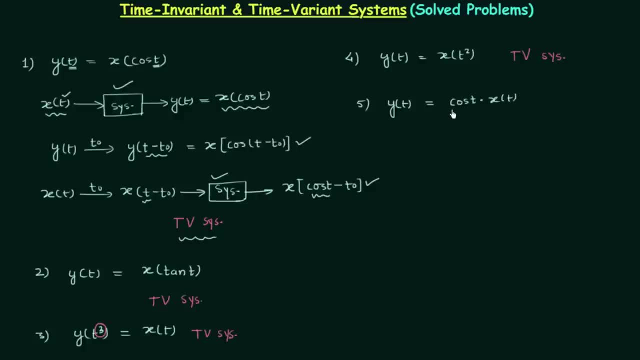 t, x, t. So in this case we have a coefficient and we have a coefficient cos t, and this x t is our input and you can see the coefficient is having t. So let's see what type of system we have in this case. first I will provide the delay to 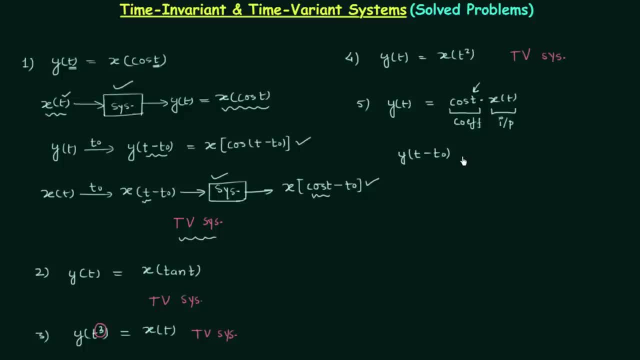 the output. So we will have y t minus t naught. So wherever you see t on this side, just replace it by t minus t naught. we will have cos t minus t naught. So x t minus t naught multiplied to x t minus t naught. 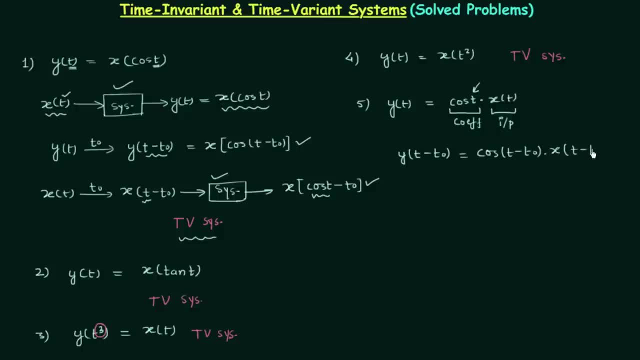 This is what we have In the second step. we will first provide the delay to the input, So we will have x t minus t naught after providing the delay to the input, and then we will feed it to the system we are having. And this time 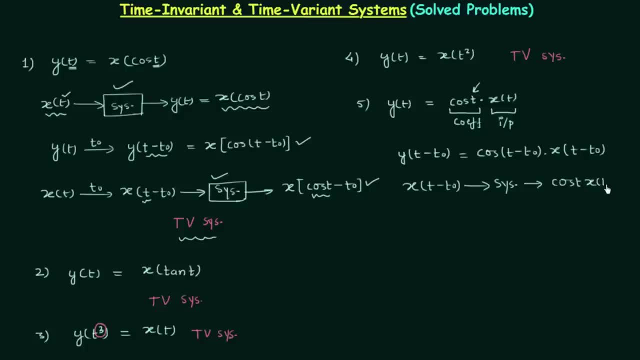 We are going to get cos t, x t minus t naught, Because if you see the property of system or the functionality of the system, it is multiplying a coefficient which is cos t to the input. The input is x t minus t naught in this case. In the earlier case it was x t and the system multiplied cos t. 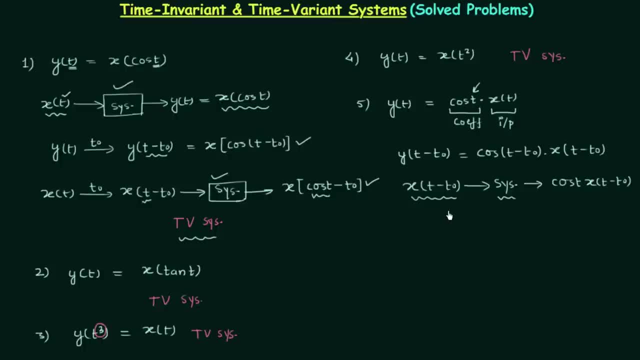 So again, the system will simply multiply cos t to the input. So cos t multiplied to the input, which is x t minus t naught. So if you compare the two outputs you will find they are not same. So we can say that the system is time varying system. 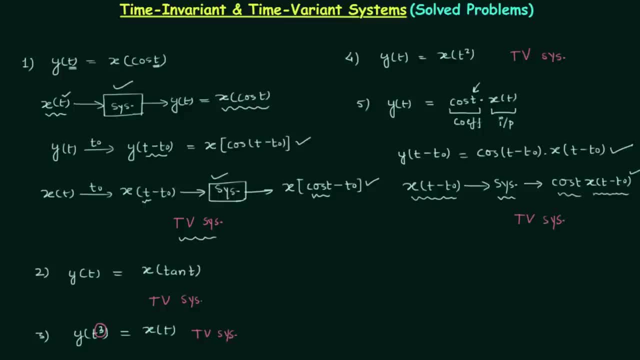 So this is what we have as the answer of the fifth problem. Now let's solve the sixth problem. In the sixth problem, output y t is equal to e raised to power minus t, multiplied to x t. Now you can see again: we have a coefficient with t. 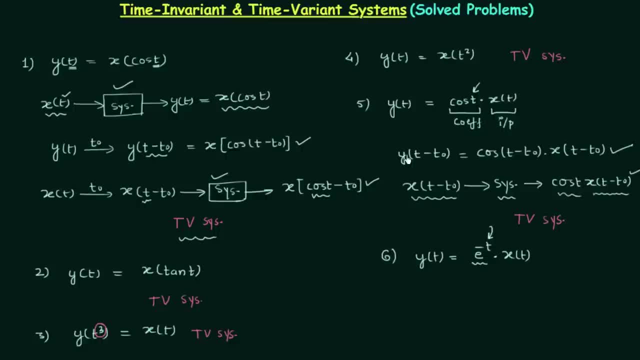 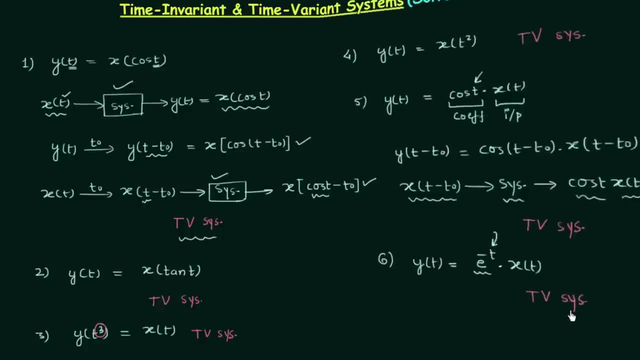 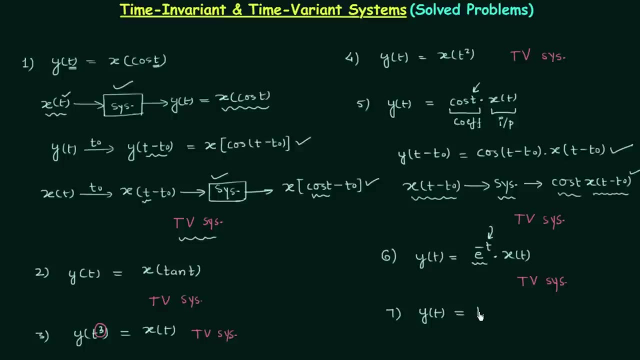 And there is time t in it. So there is no need to perform all these steps. You can directly write down. the system is time varying system. Let's solve the seventh problem. In the seventh problem, output y t is equal to 10 t plus 1 multiplied to x t. 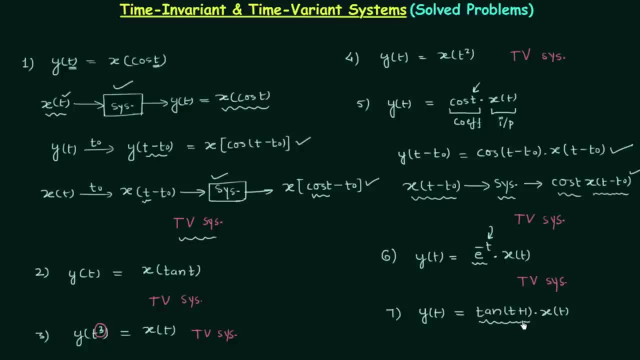 Again, we have a coefficient which is 10 t plus 1. And there is time t in it, So there is no need to perform all these steps. You can directly write down the system is time varying system. Again, we can write down the system is time varying system. 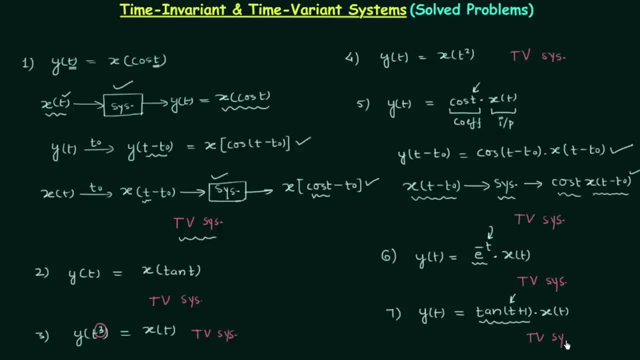 So again, this system is time varying system. So we've developed our second conclusion And according to this conclusion, when a coefficient in the system relationship is function of time, then system will be time variant. In fifth, sixth and seventh problems you can see we've coefficients and all the coefficients that we have are function of time. 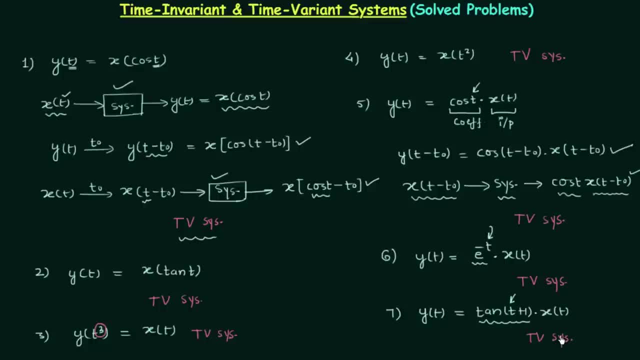 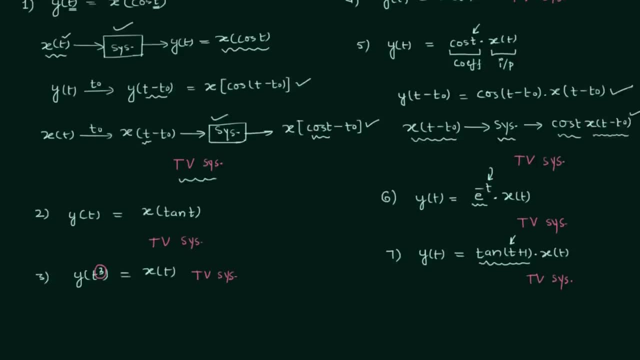 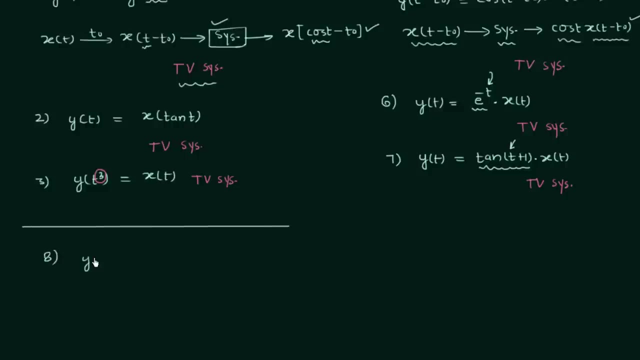 function of time. So that's it. the system is time varying system. so whenever you have such a system you can directly choose the option as time variant systems. Now let's solve the 8th problem. In the 8th problem the output yt is equal to e raised to power minus 2k xt. Now, this time we have a coefficient, but 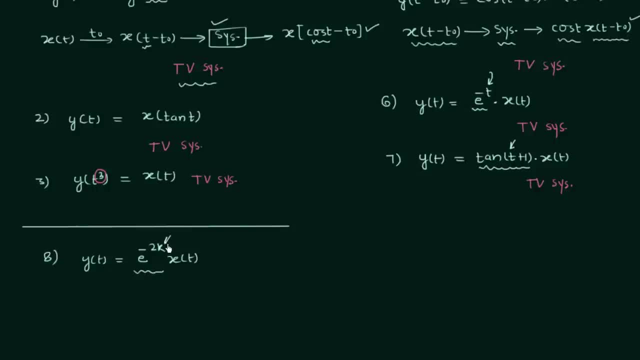 the coefficient is not the function of time, It is having k here. So this system is not time varying system, but it is time invariant system, Because if you see t here, you will find there is no scaling, and when there is no scaling the system is time variant, and when there is no time in the 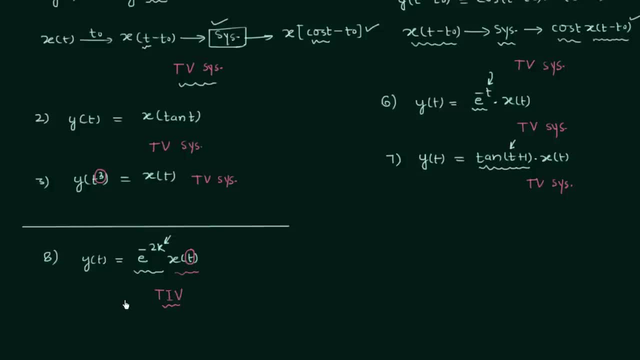 coefficient we are having, then the system is time invariant system. So the two conclusions which we have seen till now are the same. So the two conclusions which we have seen till now are telling us this particular system is a time invariant system. Let's solve the next problem, the 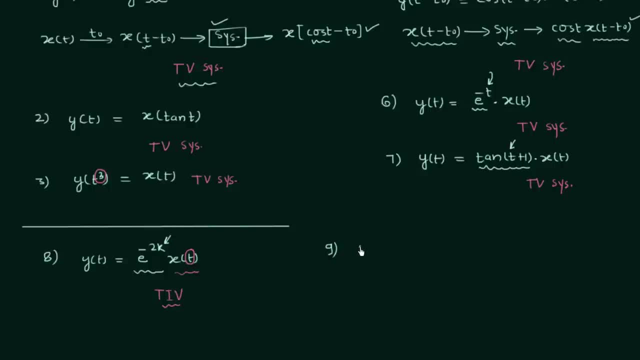 9th problem. In the 9th problem, output yt is equal to 2t plus xt. So let's try to find out if the system is time invariant or variant. I will first provide the delay to the output. We will replace. 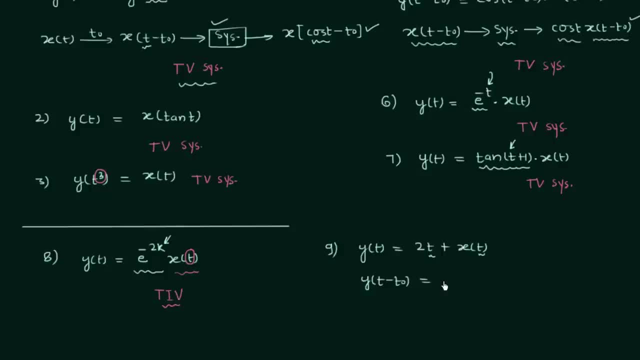 all the t's on this side by t minus 0 and we will have 2t minus 0 plus xt minus 0. now we will provide the delay to the input, we will have xt minus 0 and then we will feed it to our system and the property or the function. 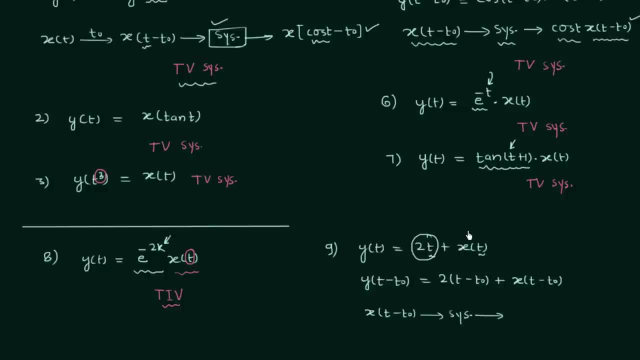 of the system is to add 2T to the input, and the system is adding 2T to the input. This time the input is xt minus not t, So the system will add 2t to our input, which is xt minus t0, and if you compare this and 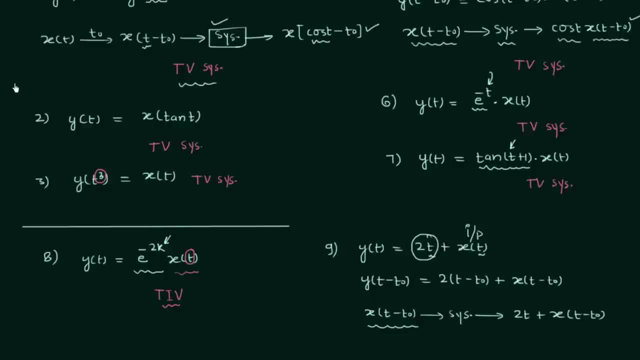 this, you will find they are not same. So the system is time varying system. This is what we have as the answer of the ninth problem, and from here you can draw one conclusion: whenever a system relationship includes any time dependent, added or subtracted term other than input or output, then the system will be time variant. 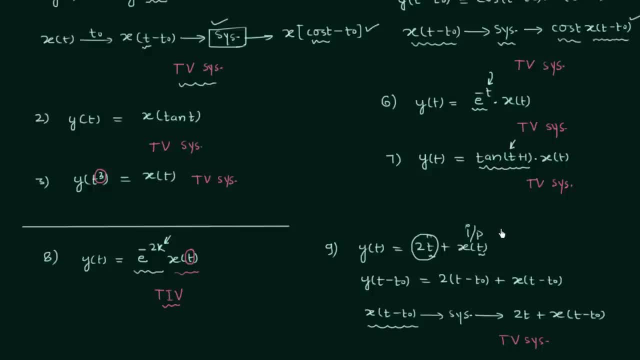 This means if there is any time dependent term other than the input or output- this is one time dependent term added or subtracted in the system relationship- then the system is going to be time variant system. So we have three conclusions in this particular lecture and I hope you will remember these. 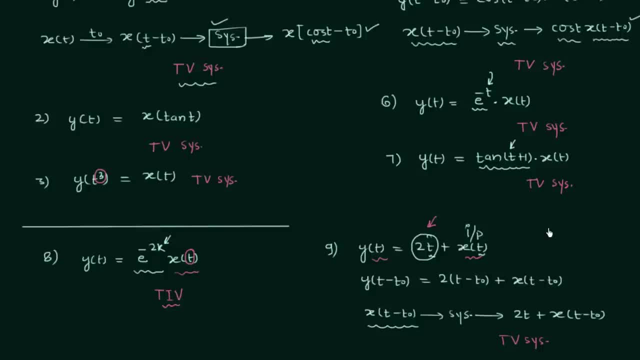 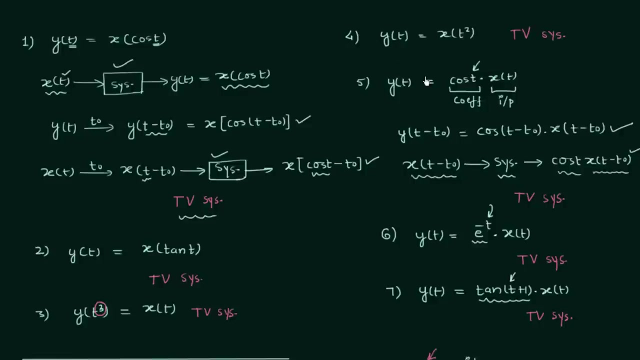 three conclusions. You can use them when you solve the multiple choice question, But when you appear in some conventional examinations, then follow the conventional way of solving the problem which we have followed in problem number 9 and also in the two problems here, in problem number 5 and in problem number 1.. 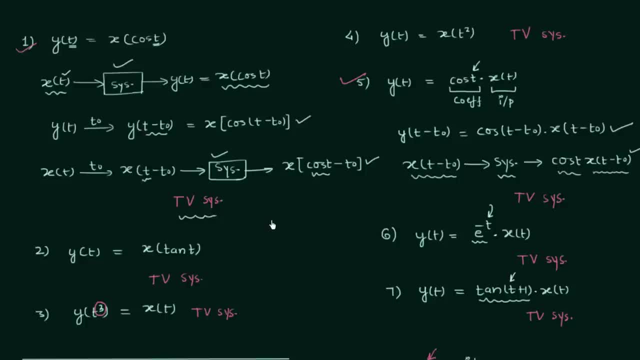 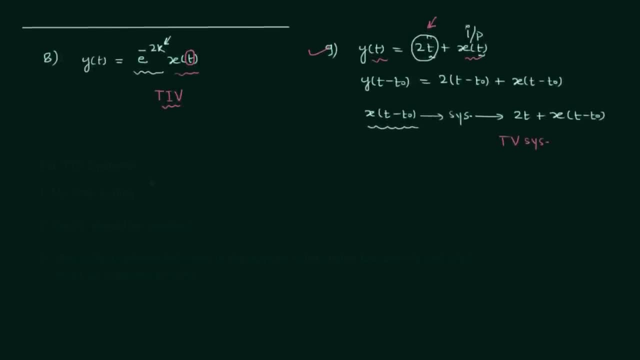 But if you use the conclusion or the direct properties, you will have your answer within seconds. I will write down all the three properties or conclusions which we have obtained in this lecture. You can see the conditions for a system to be time variant. These three conditions are very important because they are the only conditions for a